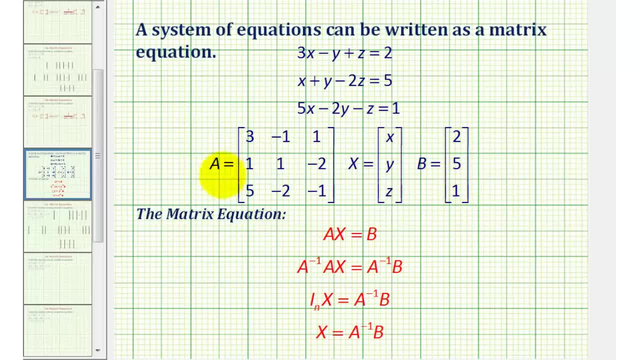 and matrix B will be the constant matrix. The elements in matrix A will be the coefficients of the x, y and z terms, The variable. matrix X will contain the variables used in the system and matrix B will be the constants or the values on the right side of each equation. 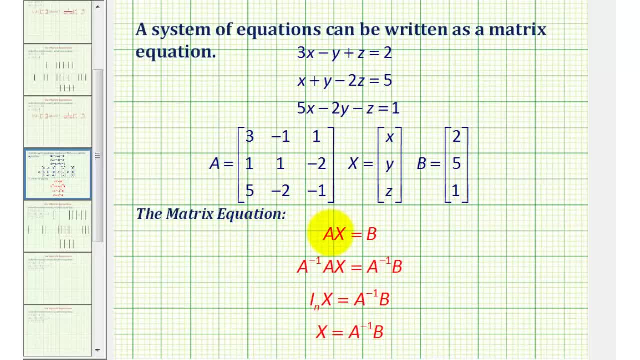 Once we have these three matrices, the matrix equation will be matrix A times matrix B, or matrix A times matrix X equals matrix B. Once we have it in this form, our goal is to solve the equation for matrix X. To do this, we'll find the inverse of matrix A, and then 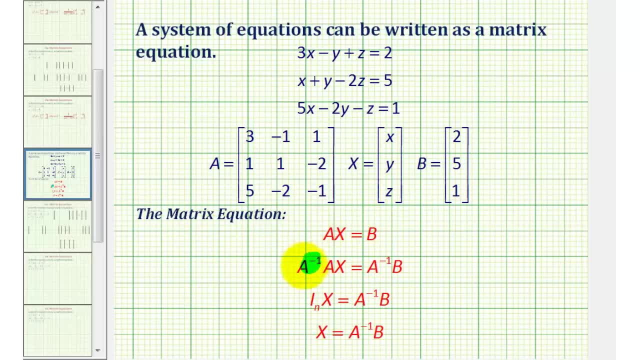 multiply both sides of the equation by A inverse. here and here- And since matrix multiplication is not commutative, this order is important- We have to have A inverse times A on the left and A inverse times B on the right. Then we should recognize that A inverse times A on 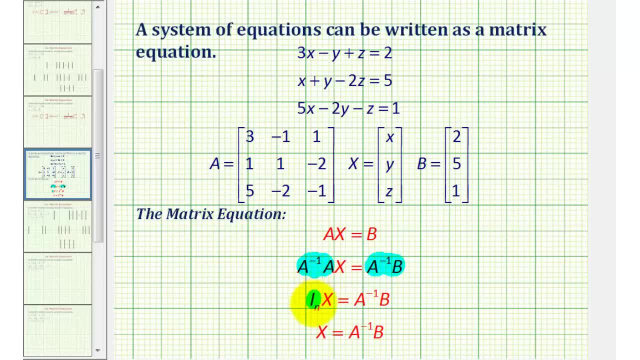 the left and A inverse times B on the right, Then we should recognize that A inverse times A is equal to the identity matrix and the identity matrix times matrix X, which is B matrix X. So, looking at the right side of the equation, A inverse times B will be the. 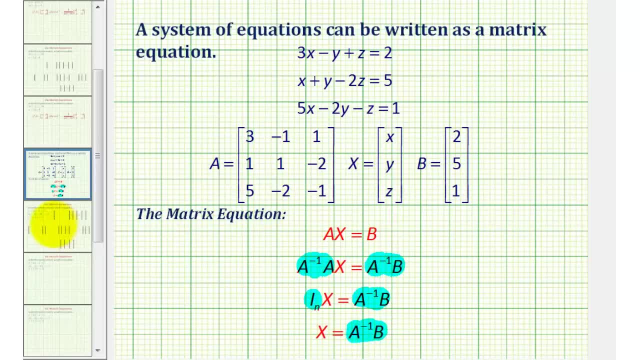 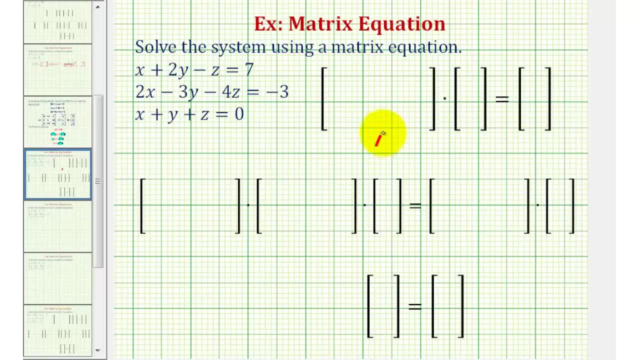 solution to our system. So, going back to our example, notice again: all the equations are in standard form. So this will be matrix A, this will be matrix X and this will be matrix B. So, looking at the coefficients, the first row in matrix A will be 1,, 2, negative 1.. The 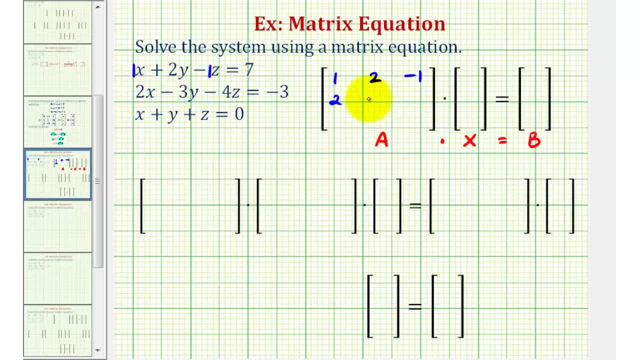 second row will be 2, negative, 3, negative, 4.. And the third row will be 1,, 1,, 1.. Next matrix: X. because we're using the variables X, Y and Z, will just be X, Y, Z. Next matrix. 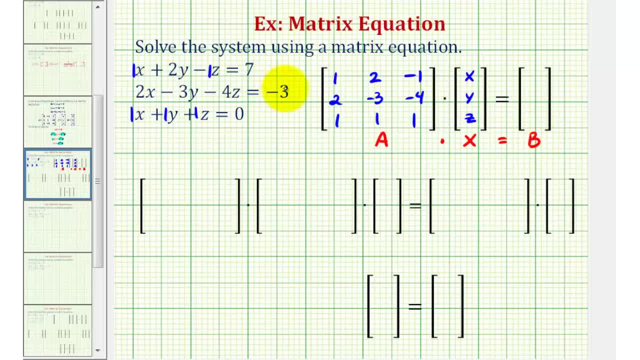 X will be matrix B, and matrix B will contain 7, negative 3, 0.. Again, our goal here is to solve for matrix X. so our next step is to find the inverse of matrix A and then multiply both sides of the equation by A inverse. So we would have: 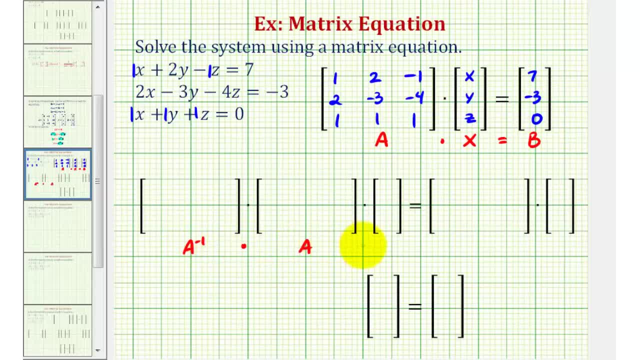 A inverse here. times matrix A, times matrix X equals A inverse times matrix B. Let's go Go ahead and fill in matrix A, X and B and then we'll find the inverse matrix. Now for this video, we're not going to find. 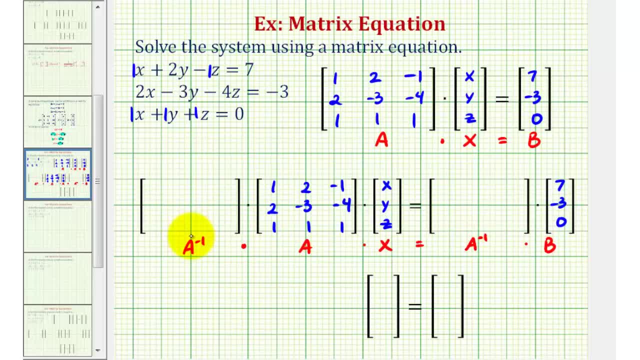 the inverse of the three-by-three matrix by hand, but I will put links on the screen to videos that will show how to find the inverse of a three-by-three matrix. We're going to go ahead and find A inverse using a calculator, So the first step is to enter matrix A. 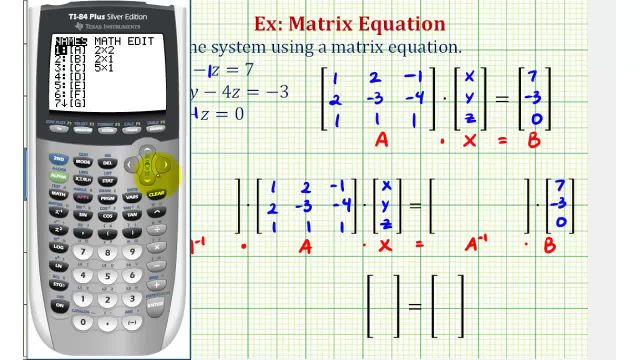 and we'll also enter matrix B. So we'll press 2nd matrix right arrow twice for edit: press enter. enter the dimensions three, enter three, enter and enter in all of the elements. It's important to double-check this. 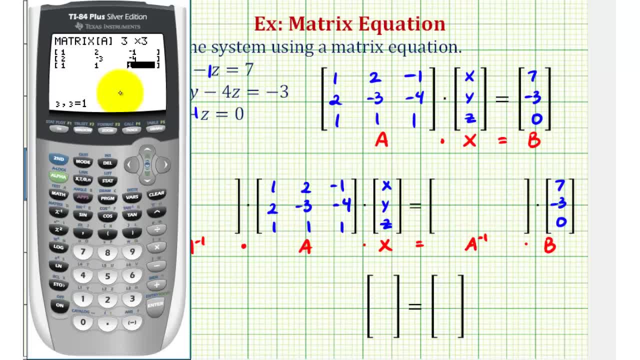 because if one element is incorrect, of course we'll end up getting the wrong answer. Now let's go and enter matrix B, So we'll press 2nd matrix right arrow to edit. arrow down to matrix B- enter. the dimensions are three-by-one. 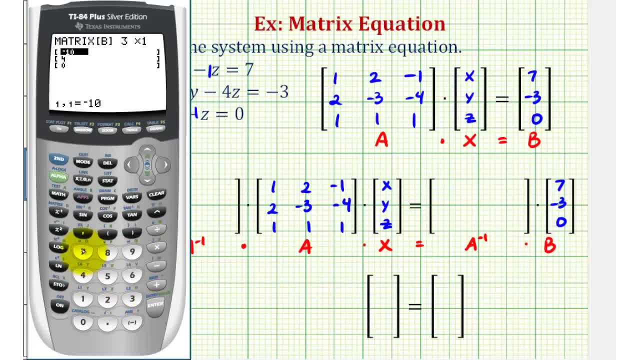 enter the elements and now we'll find the inverse of matrix A. so we'll go back to the home screen. 2nd mode for quit and then 2nd matrix, second matrix: right arrow to edit. press select matrix A. 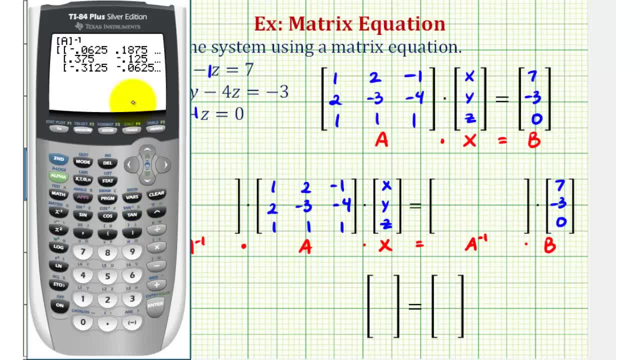 the inverse key is X to the negative one. press enter. We want to convert these decimals to fractions, so we're going to press math, enter, enter and notice how we can only see the first two columns. but if we arrow to the right, 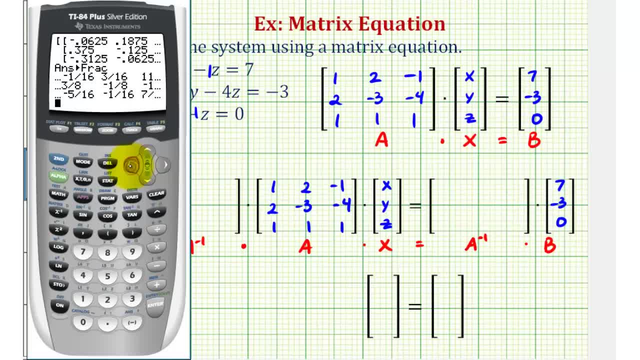 we can see that third column, So we'll go ahead and copy this down by column. First column is negative 1- 16th, which negates negative 5- 16th's. Second column is 3- 16th's, negative 1- 8th and negative 1- 16th. 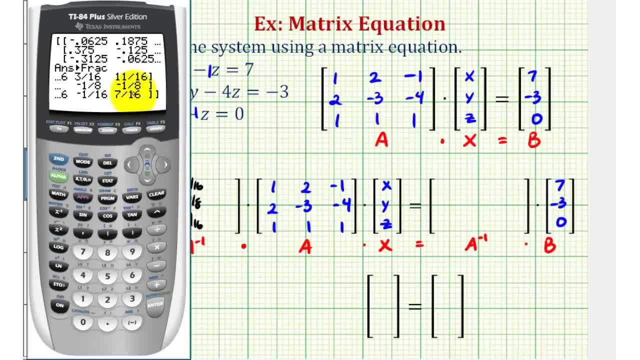 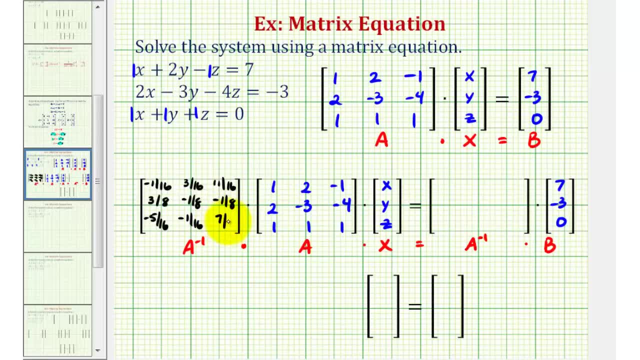 And the third column will be 11 16th's, negative 1 8th and 7 16th's, And of course we also have A inverse on the right side of the equation. Now looking at the left side of the equation,